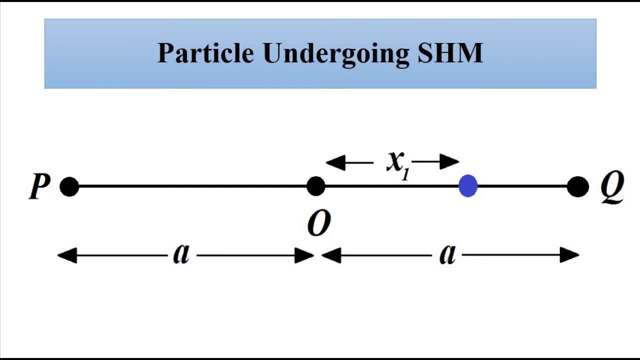 ok. It is acted upon by a restoring force which tries to bring it towards the equilibrium position, And that restoring force is always in the opposite direction to the displacement, the direction in which the oscillatory to and fro movement of a particle or an object. 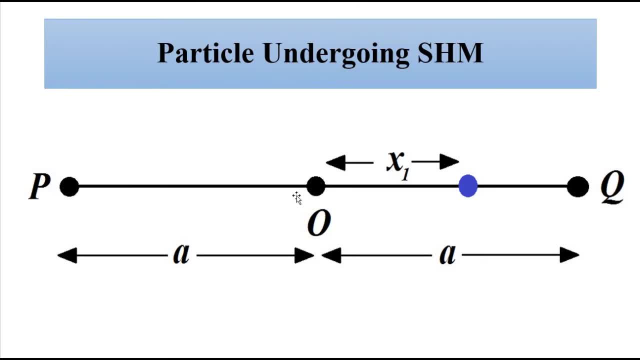 So in the previous video we discussed about the energy in simple, harmonic motion. So in this video we were discussing about the verse is also believed receiving a similar wave speed than a river speed of 0 degrees for one point to the next revolution. 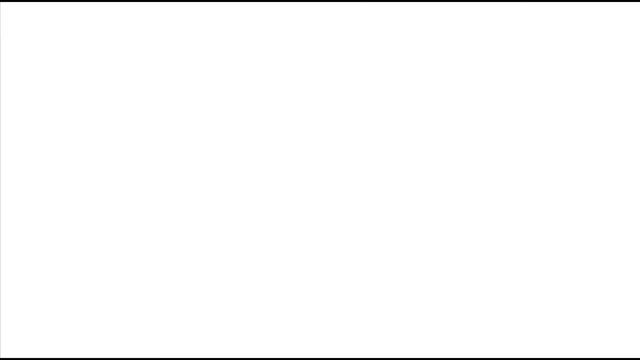 This distortion level was indeed given through, But because of the distortion domain of the oscillatory to and fro and its activation strength, we would sugar food choice. We explained. you can use this position system in the next video to write. because these surfaces they are called oscillatory Left corner. 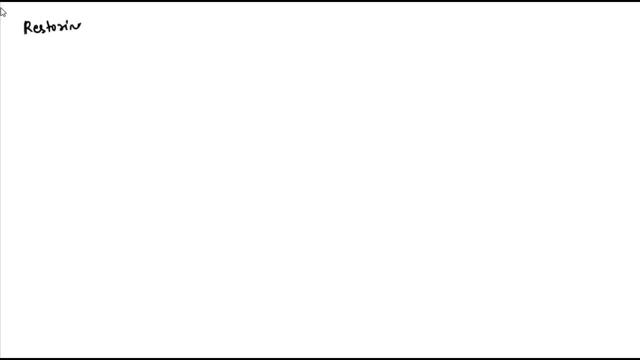 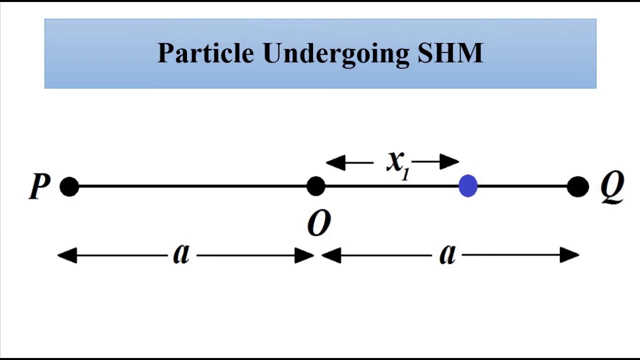 See to the right force. it gives rise to one component of the energy and simple harmonic motion which is called as potential energy, potential energy of the body undergoing simple harmonic motion. Now, as the body is in movement, it has certain velocity and because of that velocity there. 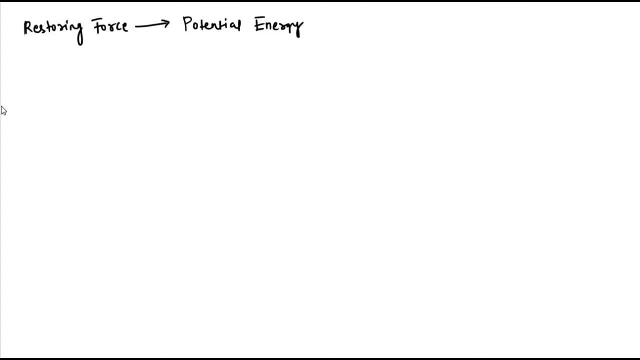 is another component because of the motion of the body, the body in SHM, simple, harmonic motion- Because of its velocity, Okay, It has the second component, which is kinetic energy, And these two energies are there, are considered when we are, you know, considering the simple. 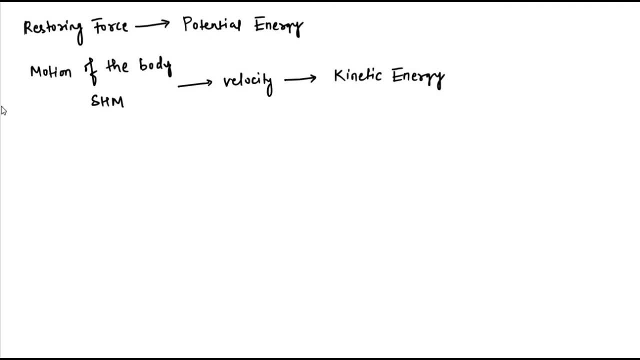 harmonic motion and this potential energy and kinetic energy. It gets continuously interchanged from one to the other, while the total energy content of the signal it is fixed Okay, As the body or the object it undergoes: simple harmonic motion, potential energy and kinetic. 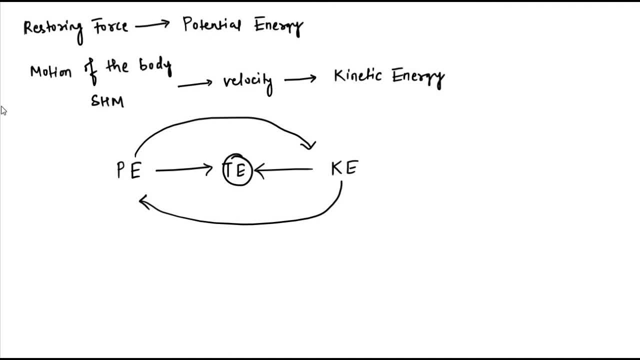 energy, it continuously gets interchanged, Okay, But The Net energy, it is always constant. The law of conservation of energy: Okay. Energy can be, you know, transferred from one form to another, but the net energy, energy can neither be created or destroyed. 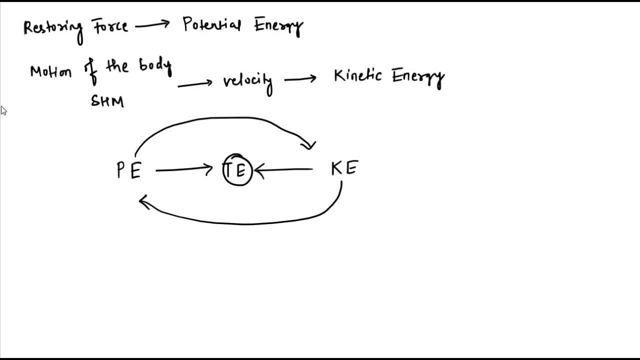 So the same principle here. Now we know we have already derived that the acceleration of an object or a body undergoing simple harmonic motion, it is given as this, Okay, Instantaneous displacement- and the angular, we can say angular- frequency, considering the motion or the SHM motion. 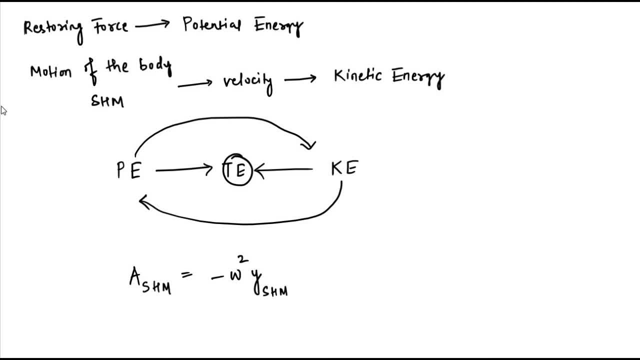 Now, because of this acceleration, the restoring force which acts on the body, trying to bring it towards the mean position. it is given by mass multiplied with this SHM acceleration, Okay, Which is given by minus m omega square y SHM. This is the restoring force, and it is also given by minus k y SHM, where this is the constant. 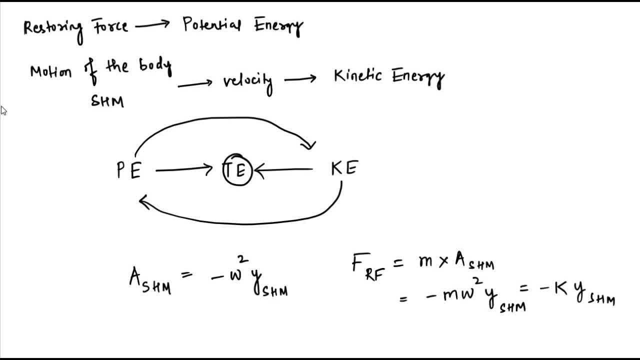 this minus m omega square. Okay, So now, Okay, So Under the influence of this restoring force. Okay, Under the influence of this restoring force. suppose the particle. okay, under the influence of the restoring force. in the opposite direction, let us say a particle it undergoes, let us 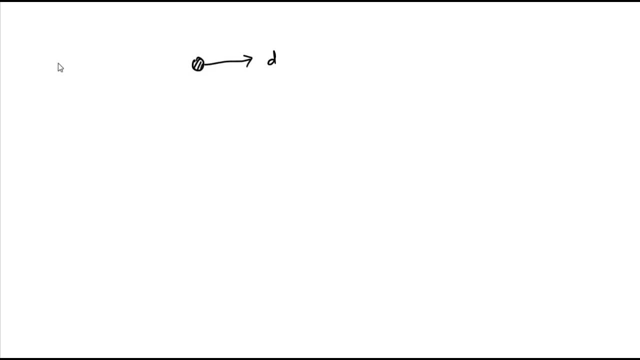 say displacement, this much by a margin of d? y. Okay, This, This is registering force and this restoring force acting in the opposite direction, Okay, Okay, So alright. Therefore, it undergoes displacement d? y, small displacement d? y, So alright. 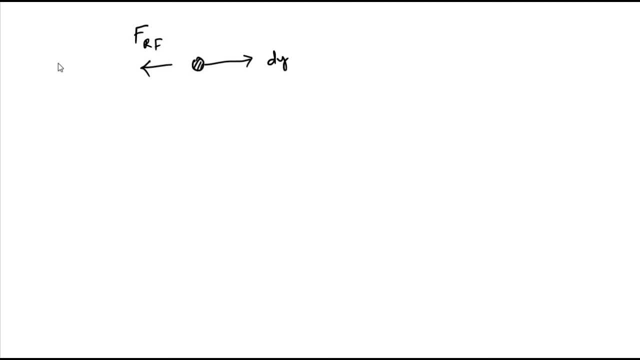 So. so let us assume that the displacement d, y, also y, was 2 times僕 pow изуч dimensions of mass multiplied by 6, q, i, d, y. We know that this logistics unit in principle is. we know that in the case of jak paralleleks. 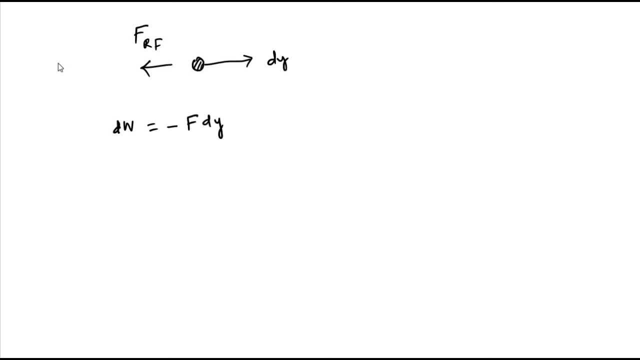 with M graph. here you can see that project will be Sterling. Okay, We can simply double сложно and distribute r and z as inverse. We can also multiply each theta, And then all this from the crediticação contribution. Okay, opposite to FRF. ok, F is in the direction of dy, F will be in this direction. restoring: 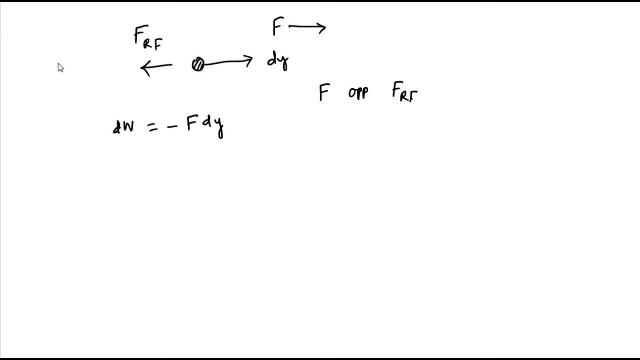 force is in the opposite direction. So this F is opposite to FRFs, but equal in magnitude. So it is given by minus ky dy, because restoring force is minus ky ky SHM. We are simply writing it as ky ok. So it is the same thing: ky SHM and this ky. they are the same thing Instead. 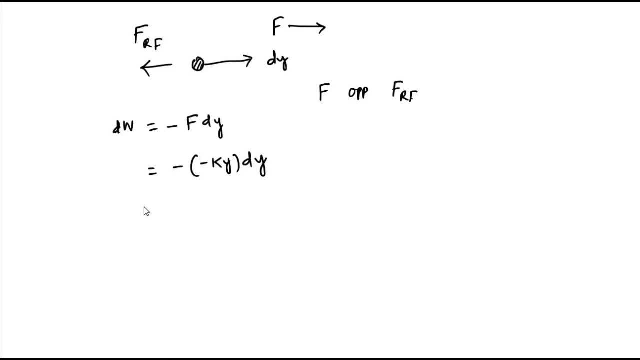 of y SHM. I am simply writing y, So this is given by dw, is equal to ky SHM And the total work done is integration of dw. and this is for the total displacement which is given by one half ky square, integration of ky dy. this one half ky square, So this. 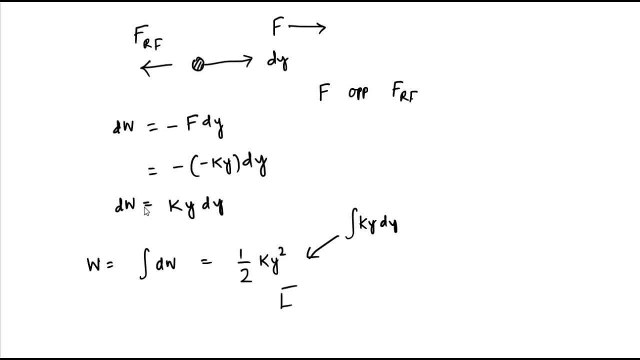 is the potential energy. This is the potential energy. So this is the potential energy. So this is the potential energy, potential energy. ok, So the potential energy or E p of a particle undergoing SHM is given by 1 half k y square. or, if we just refine it a bit, this instantaneous displacement in: 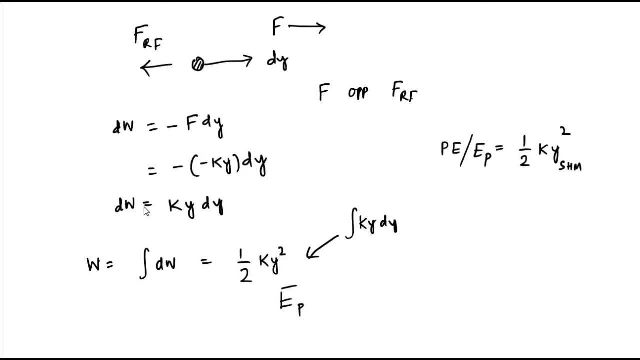 simple harmonic motion. So do not get confused with y and y SHM. ok, they are the same thing: instantaneous displacement in simple harmonic motion. Now, if we include the constant k in it, in its original form in terms of the mass and angular frequency, it will become: 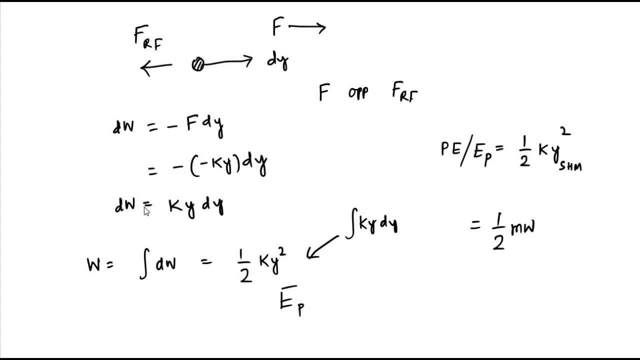 1 half m omega square, y SHM square. this, This is the potential energy. next is the discussion related to kinetic energy. Now, suppose the velocity of the particle in SHM. we have already derived in the important parameters and we got the value as omega a square minus y square or y SHM. These are: 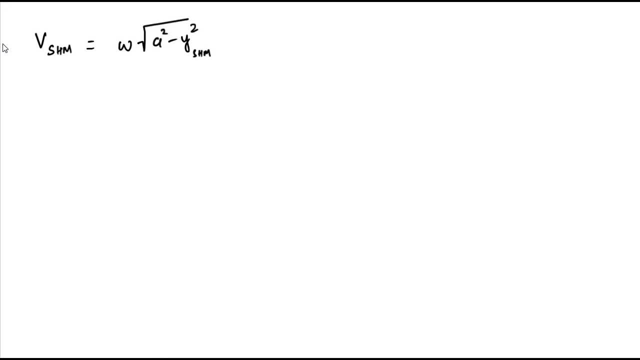 h m square. let us call it ok y and y h m. they are the same thing, but here, just for your understanding, I am writing it in this way: where omega is the angular frequency, y h m is the instantaneous displacement, a is the amplitude, the maximum displacement from the 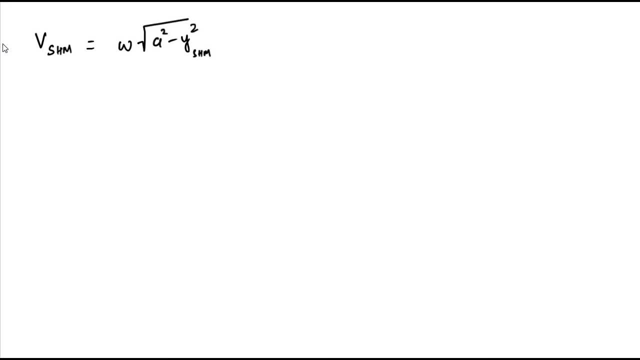 mean position. So please watch that video related to important parameters, where we have derived the expressions for displacement, the general equation, then time period, frequency, velocity, acceleration, everything. So we know that the kinetic energy of any object with certain velocity is given by half m v square, So here it will be half v s h. 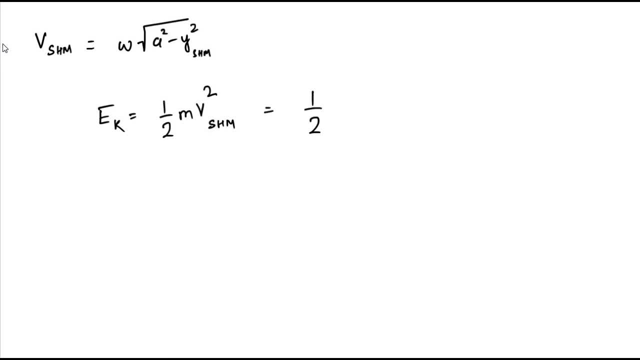 m square. So it will be 1 half m omega square, a square minus y, s, h m square. this is the kinetic energy. So this is the expression of kinetic energy: 1 half square, a square minus y, simple harmonic motion square, this. So we have got the expression for kinetic energy and we have got the expression. 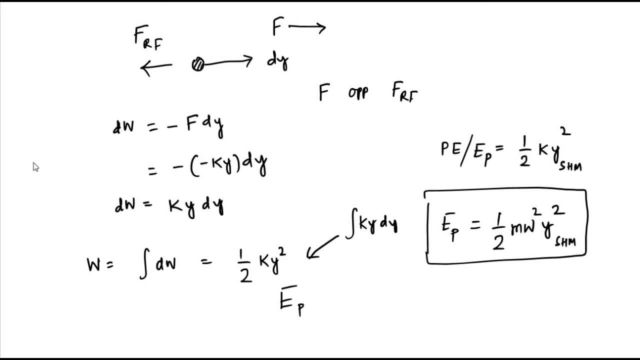 for potential energy. ok. So now the total energy. total energy is kinetic energy plus potential energy. ok, So that is for the potential energy. first, 1 half m omega square, y square. So this is the energy as can be defined by half m v s h m square, y square, ok, or y s h m square, let us call it again. 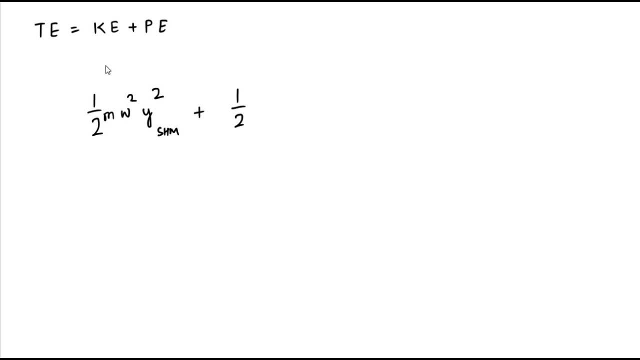 do not confuse with y and y s h m. they is the same thing. this is 1 half m omega square a square minus y s h m square. this is the kinetic energy. So here you can see, there will be one half m you omega square y s h m square. this is here minus 1 half m omega square y. 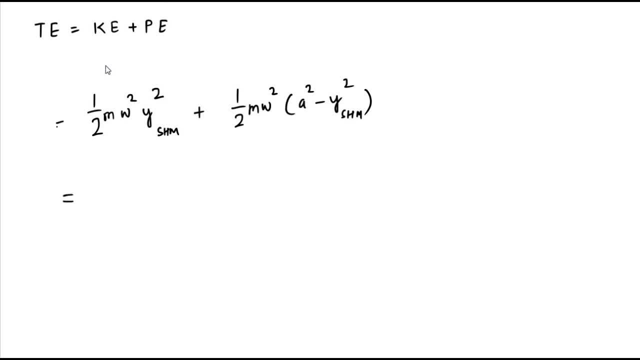 s h m square, So mutual displacement. here you can see two meters square minus y s h, y s h m square, And this is also the funded vi方面. here it is sigma equal to one half. get cancelled and we will have one half m omega square, a square. this is the total energy. 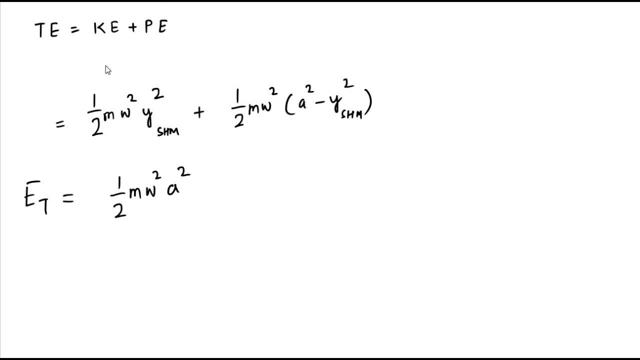 of the signal. ok this. So, as you can see, at any instant, in the simple harmonic motion, the total energy, the net energy, is always fixed and it always gets interchanged between kinetic energy and potential energy. ok, So here for a particular object, ok, a. 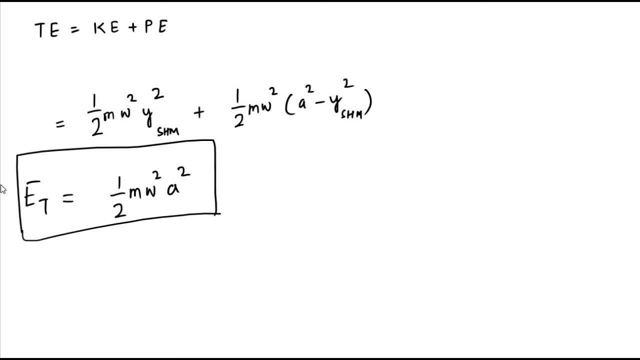 particle in SHM mass is fixed. ok, maximum amplitude is fixed and the angular frequency is fixed. So the total energy, the net energy, for the entire duration of SHM will be fixed, but it will get interchanged from one form to the other. 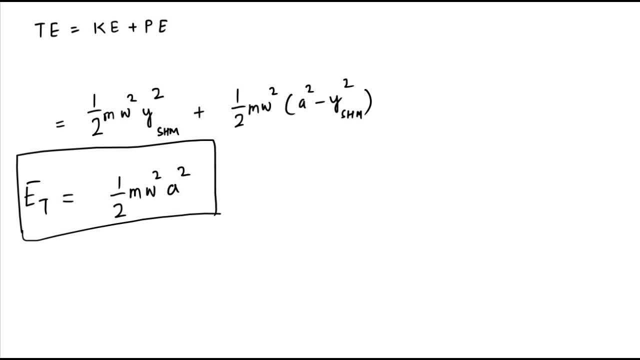 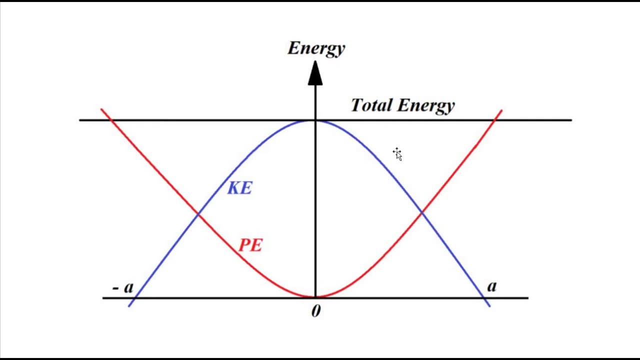 Now here, if we want to represent the energy of a particle in SHM in graphical form, it will be like this: So here, if you notice the blue plot, the both kinetic energy and potential energy are graph versus displacement, the energy, kinetic energy and potential energy. 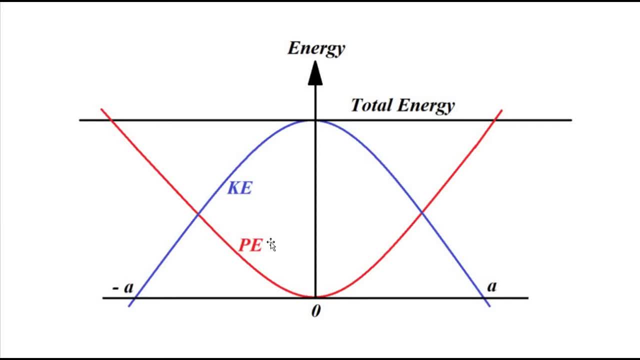 versus displacement. it will always be in the form of a parabola: centered around y is equal to 0. ok, So this is displacement. ok, this is displacement and this is energy. So here is a parabola: centered around y is equal to 0, this blue one is for kinetic energy. red. 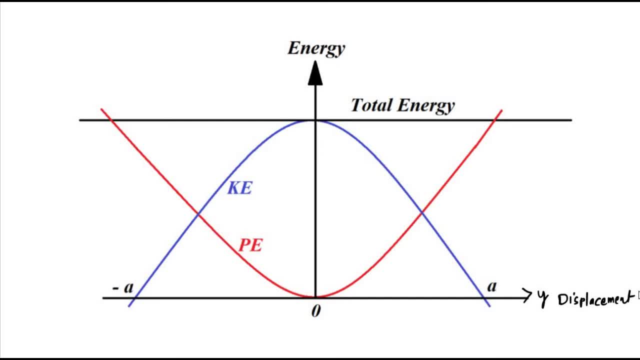 one is for potential energy and the straight line parallel to the displacement axis. this is for the total energy. ok, So here the kinetic energy. as we have already derived the kinetic energy expression, the kinetic energy will always be like this: one half m omega 1.. 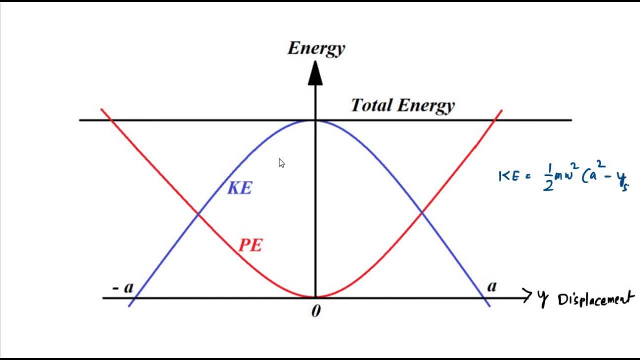 and potential energy. that is equal to one half m. omega square y- instantaneous displacement. y s h m- whole square. ok, So this is the graphical representation of the energy content of the signal in simple harmonic motion. Now, here at y s h m is equal to 0 at the center position. 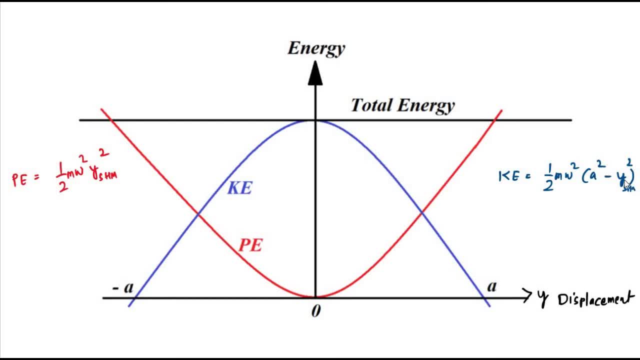 or the equilibrium position, Kinetic energy will be just. we substitute y, s, h, m with 0 and will become one half m omega square, a square, ok. And when this will become 1 half m omega 0 at the equilibrium mean position, potential energy will be 0, as see here, it will be 0 and 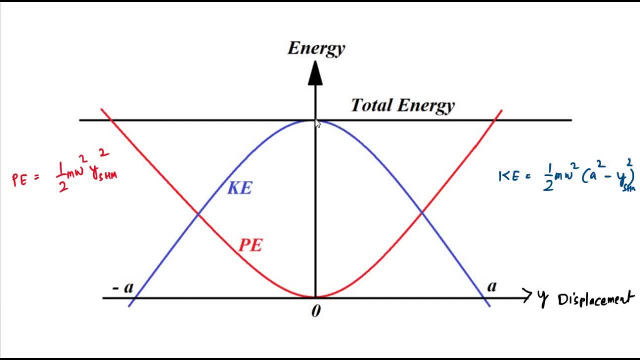 will be maximum at the equilibrium position. Kinetic energy will be maximum at the equilibrium position. potential energy will be minimum 0 at the equilibrium position. At the extreme positions, y is equal to plus minus a. if we substitute here a kinetic energy, y, s, h, m with. 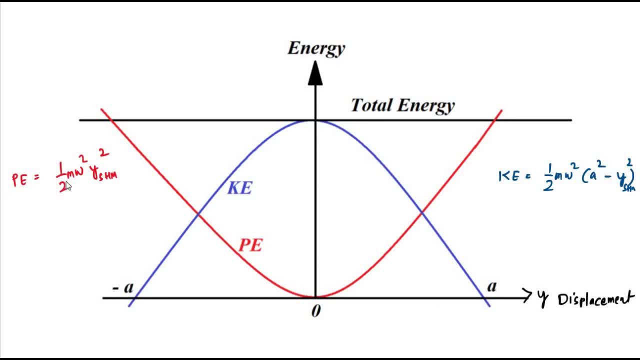 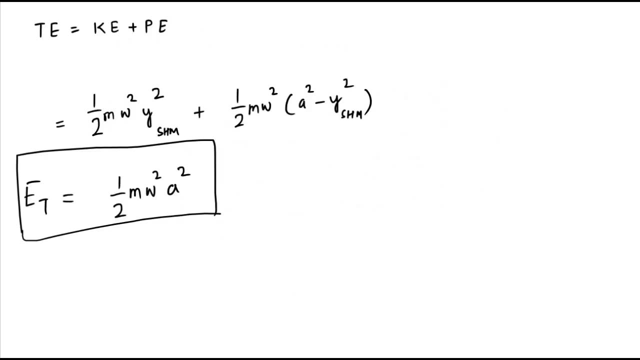 a, it will become 0, kinetic energy is 0 at the extreme points And here, at the extreme points, potential energy is maximum, equal to the total energy, the maximum energy, the total energy here, which we derived. ok, So this is the whole thing for the entire duration of the simple harmonic.